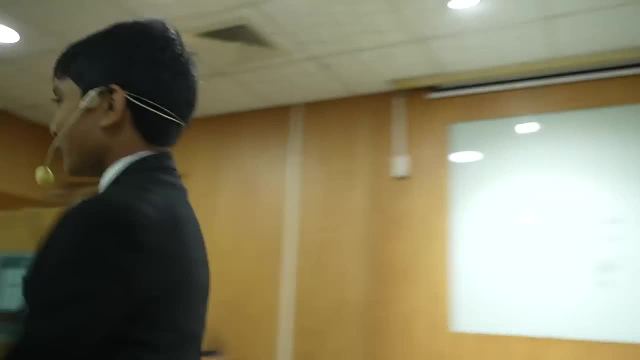 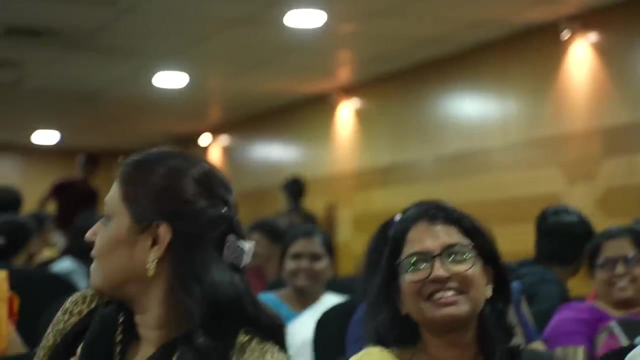 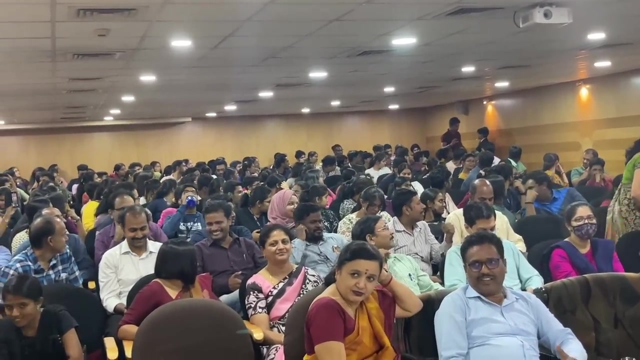 Can someone raise their hand? Oh, I'm just going to come over because I can't hear you from all the way back. Yeah, Oh, same person. First, reflective index. We can find the reflective index. Reflective index equals to one upon sine C, sine C, The C is the critical angle. 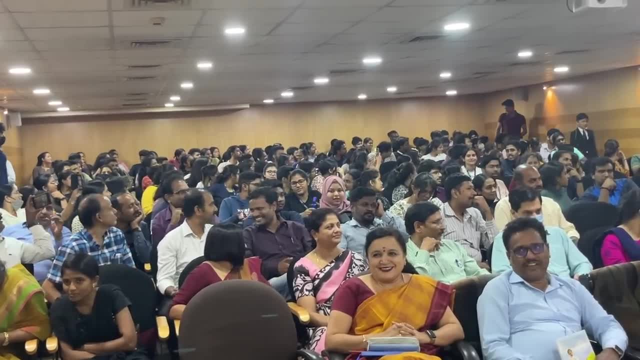 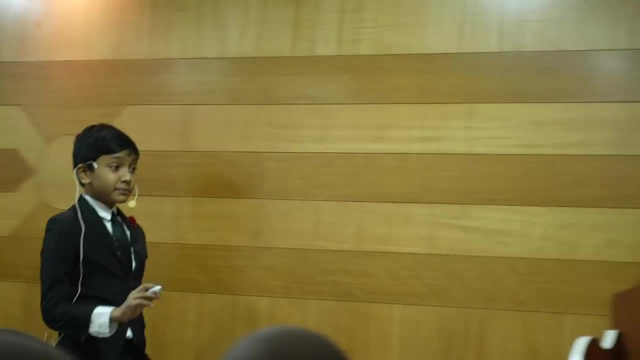 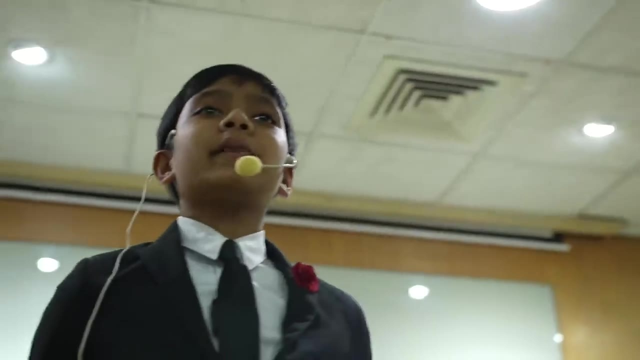 Okay. Well, it does have something to do with the index of reflection. It does have something to do with the index of refraction. so I guess you did better than last time, but Louder. I heard something: N2 cannot be greater than N1.. 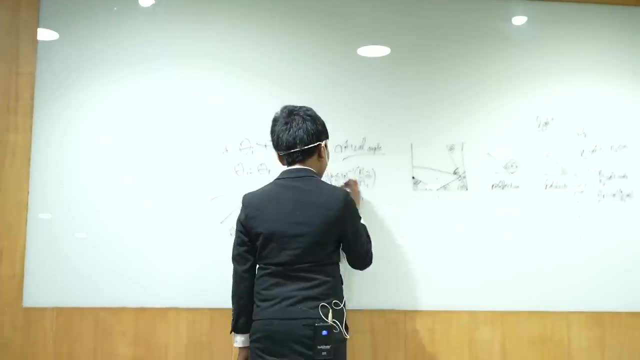 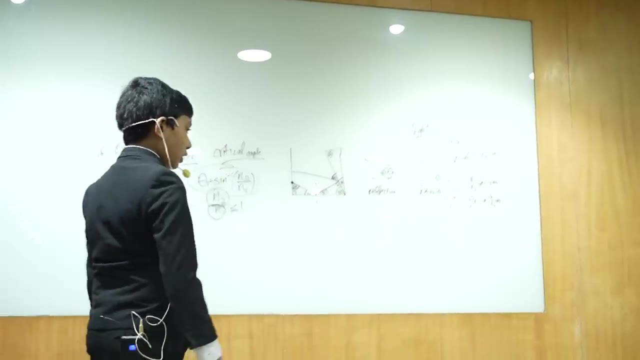 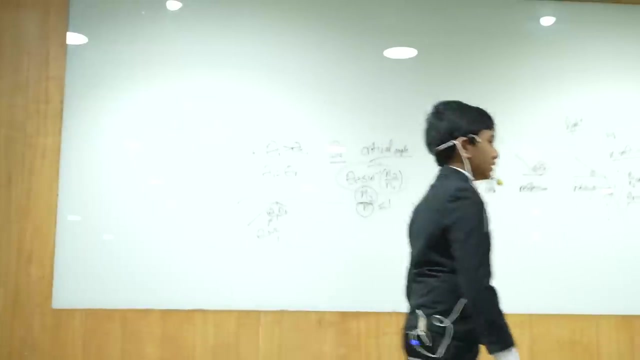 Good, Good, Finally, A good answer regarding something mathematical, Finally. So now let me give you a geometrical problem that, again, no one will probably try to solve. Regarding the critical angle: Okay, I probably don't need this one, so there's enough space. 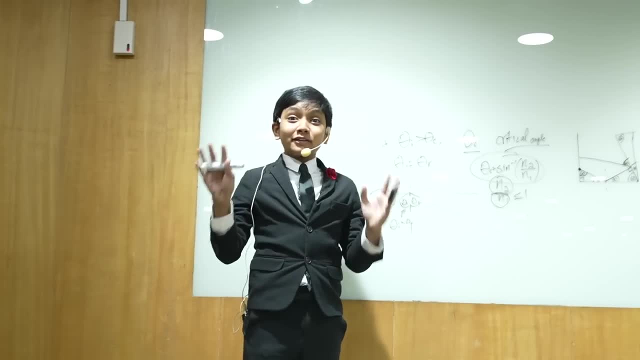 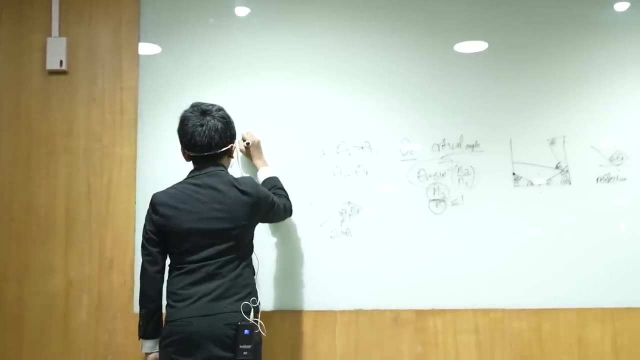 So okay, And I know you guys are freaked out by anything with more sides than a square, but let me draw a. let's not draw over here. let me draw a hexagon. I know this has you guys freaking out. 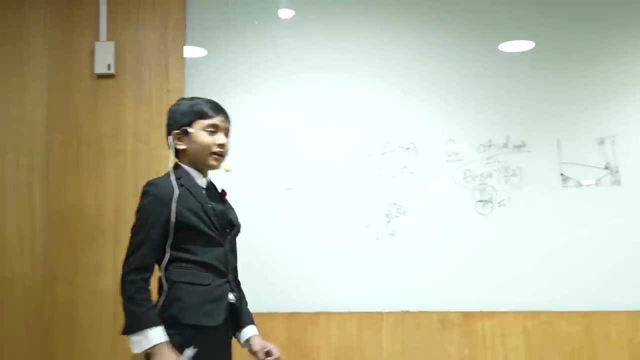 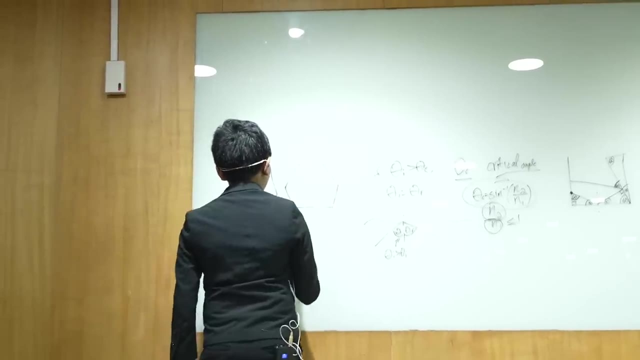 I know you're trying to remember the degree measure of a regular hexagon right now, but don't worry, It's going to be fine. It's not going to be fine, Okay, Okay. So let's say we have a hexagon half full of water and half full of air. 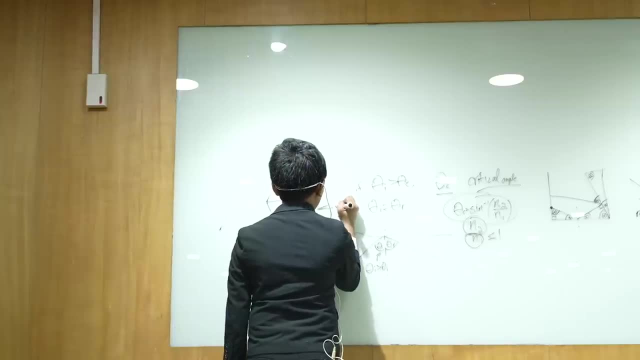 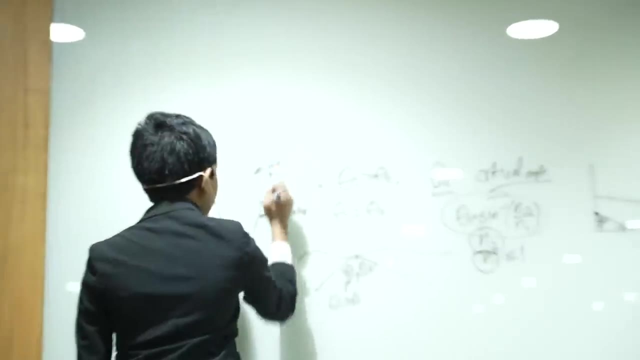 And since you guys and for you guys, the water is on the bottom because gravity works, So this is water and this is air. Since you guys probably also don't remember the index of refractions of those, I'm going to write them down too. 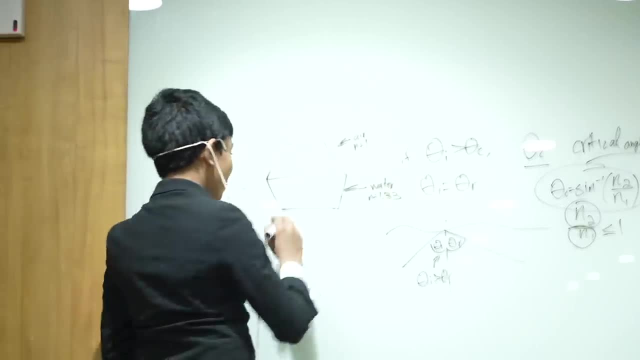 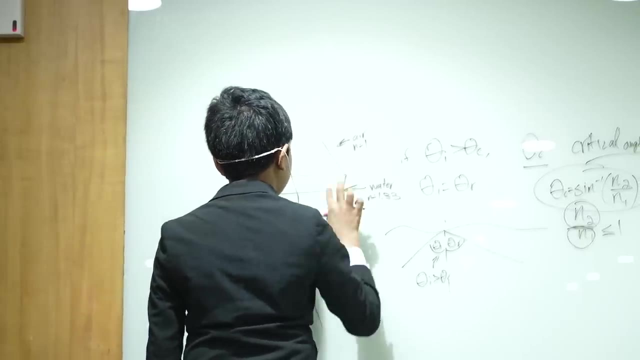 Alright, So now I know you guys don't know what this is, but let's take the midpoint- yes, the midpoint- and then the light ray is going to depart straight over there And then it's going to bounce off here. 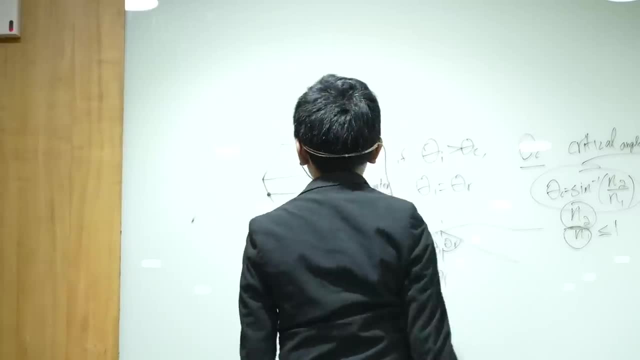 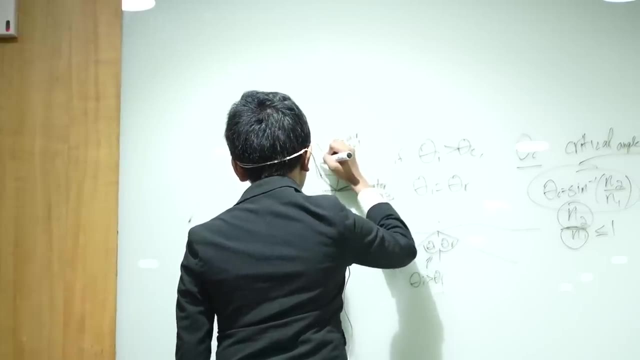 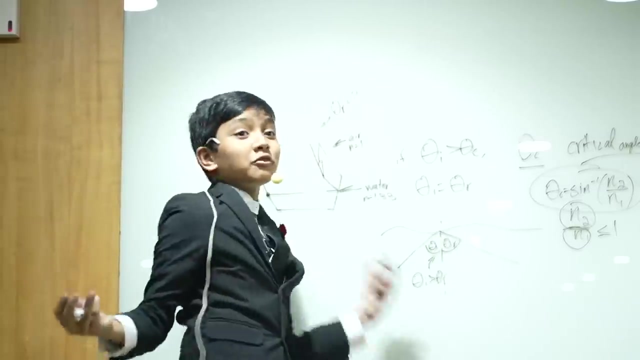 It's going to reflect, so I'm going to draw- try to draw that- And it's going to refract over there. So I want you guys to find out what this angle right here find this angle. Anyone want to come up here, Do it? 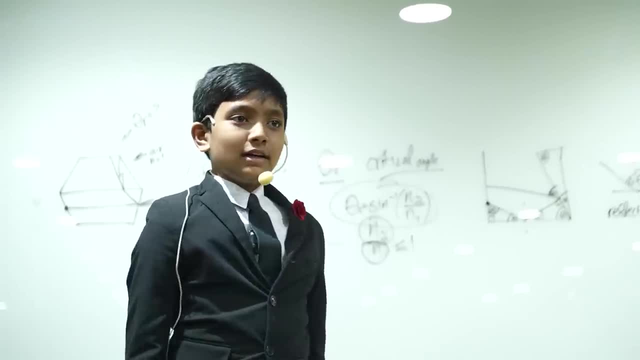 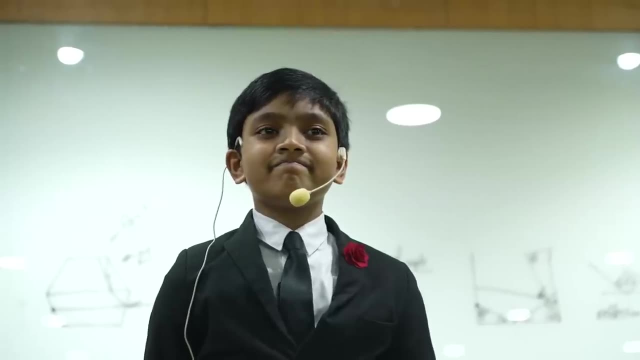 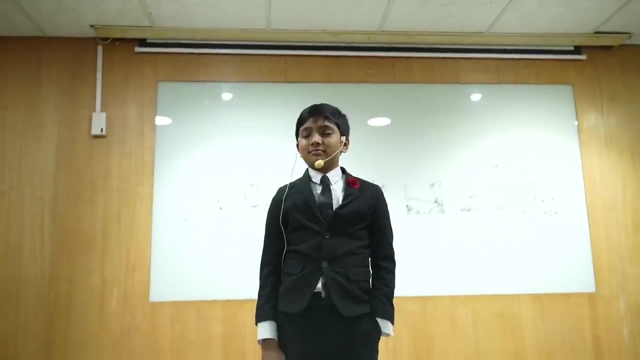 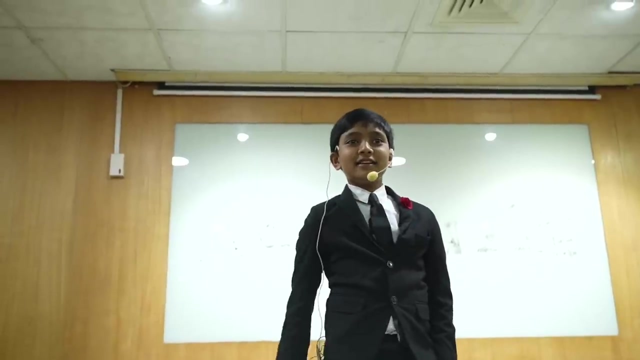 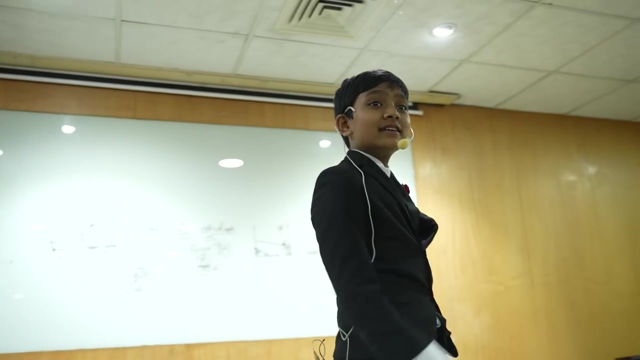 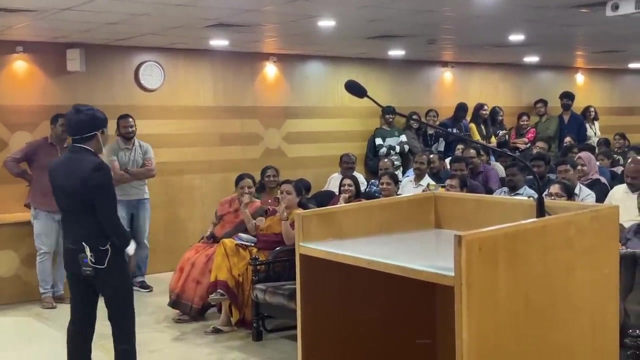 Anyone. Take out your notebooks and your pens. Do it on paper. Come on guys. Okay, good, I see someone with a notebook and a pen. At least they know what they're doing. Don't shake your head. I need nods. I need nods. 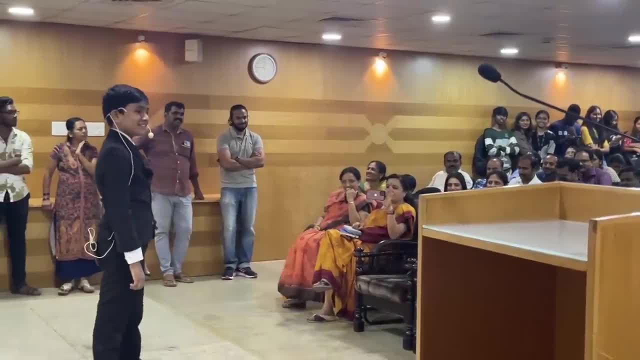 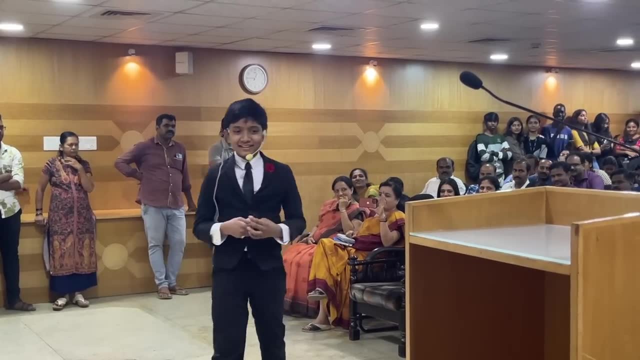 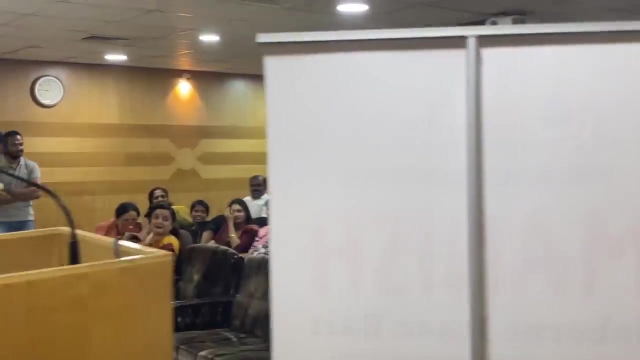 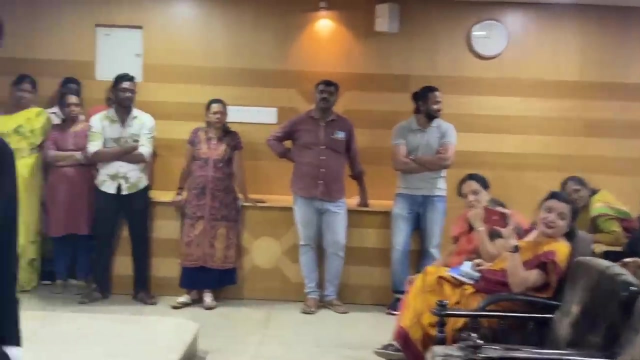 Someone Just come up to the board Please. I'm a biology person. I'm a biology person. basically I don't understand, But I can only know. probably A is the kingdom medium and water is the denser medium. 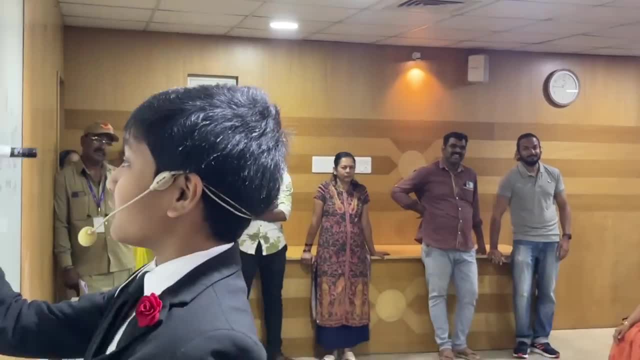 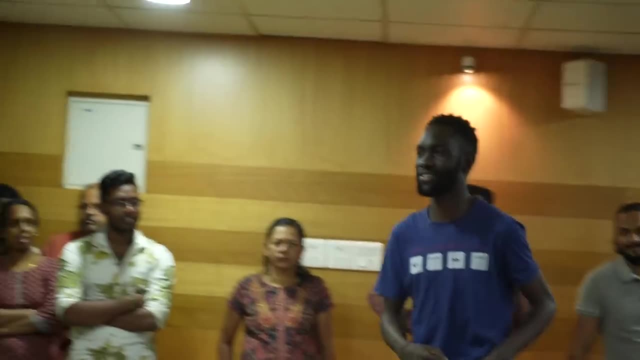 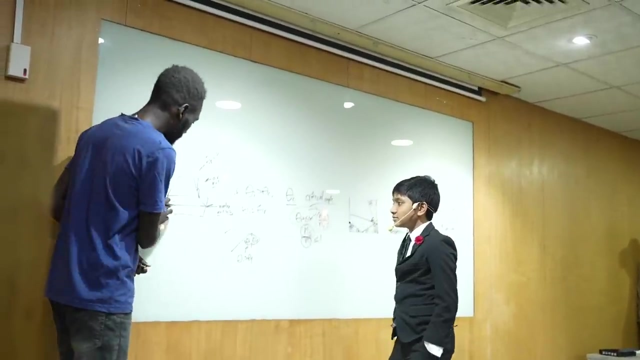 That's what I understand, Okay. Well, the index of refractions already told us that. Sure, Just give me an idea of how to do an answer. Anything better than a wrong answer is good at this point Here. Okay. 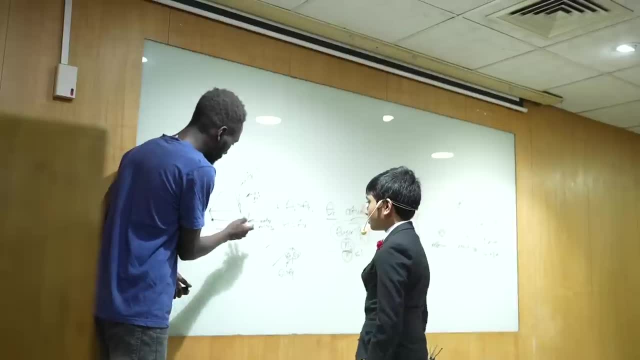 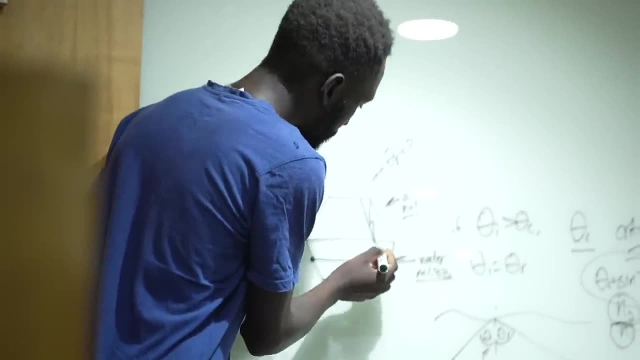 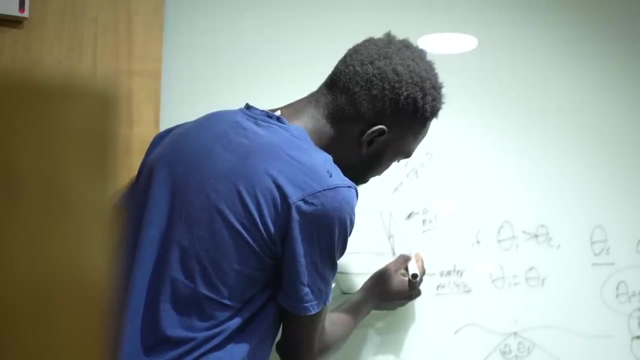 So this is water? right, Yes, that is water. Okay, so this angle is equal to this angle and these two angles are equal. Okay, Yeah, and then we have, since this is straight, we have here: this is 90 degrees. 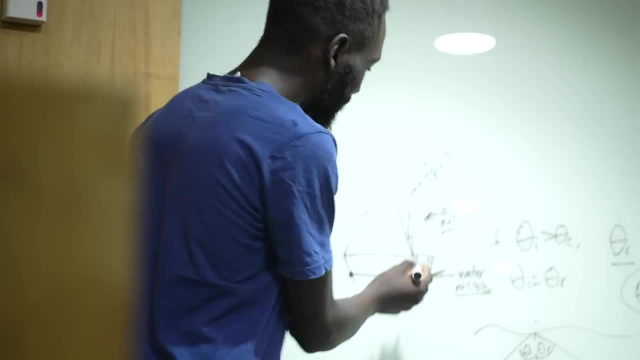 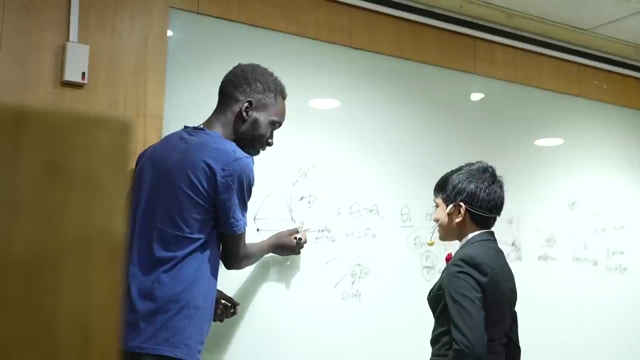 so you can do this angle here, Right, Because this is an oil height. Yeah, these two angles are equal. Then here we have 90 degrees. Sorry to tell you, bud, but the degree measure of one of these is 120 degrees. 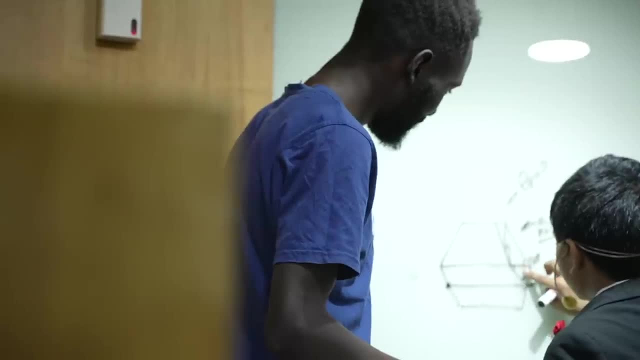 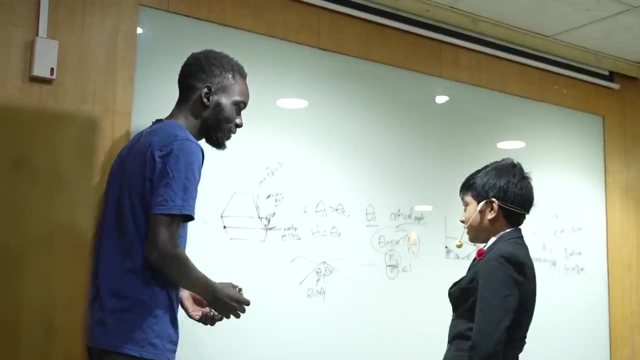 and since you're splitting it straight down the middle, this is going to be a 60 degree angle. Okay, So we can find this, since we know this too. Okay, Yeah, then we can use it to get this angle you want. 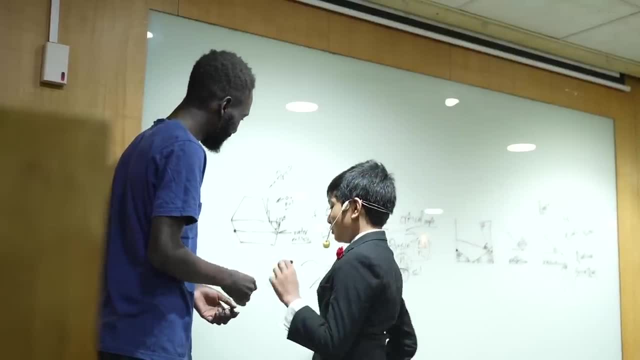 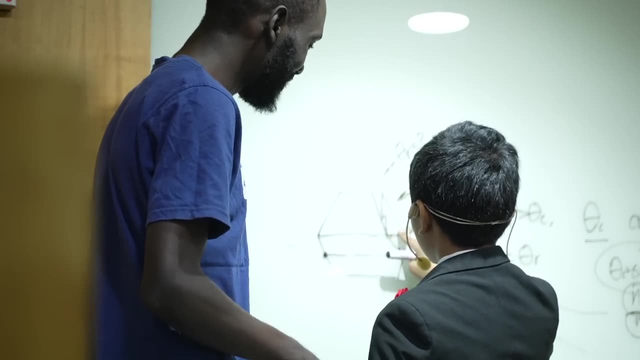 Yes. so I don't know, Maybe it was better than some of the answers you guys would have provided if I called you up to the board. but let's actually do the true solution. You can sit back down, It's okay.